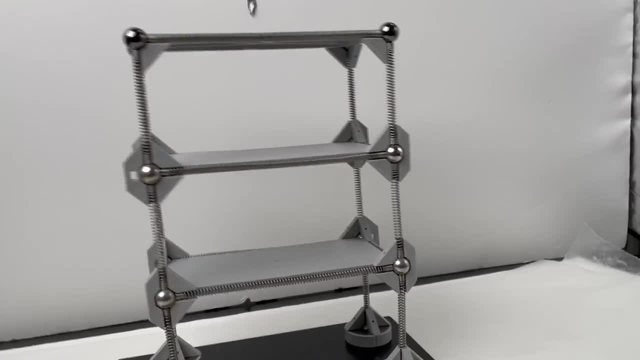 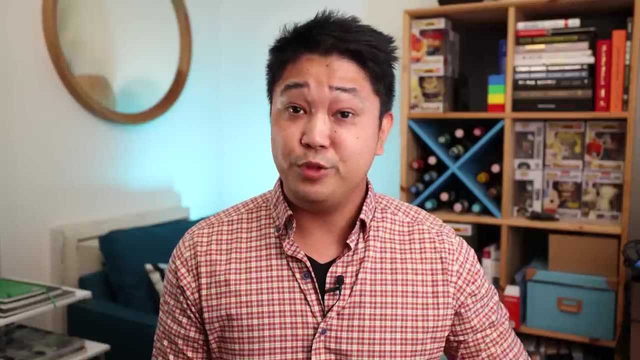 I'm stiffening the joints up on this Mola model kit. It's a kit that was designed to simulate the structural behavior of buildings and stick till the end. If you want a 20% discount on these Now, let's put it through an earthquake: It's still standing. 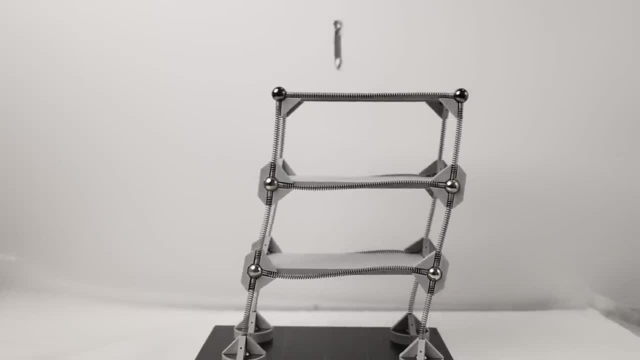 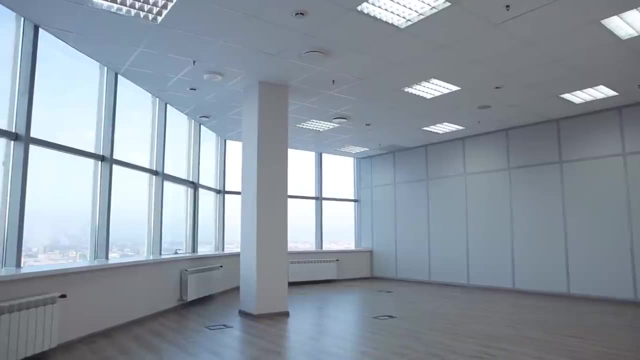 but it does seem to wobble and deform quite a bit, And that's one of the cons of using a moment frame system, along with it not being the most economical solution. but architects love them because you don't have any walls or braces in the way. 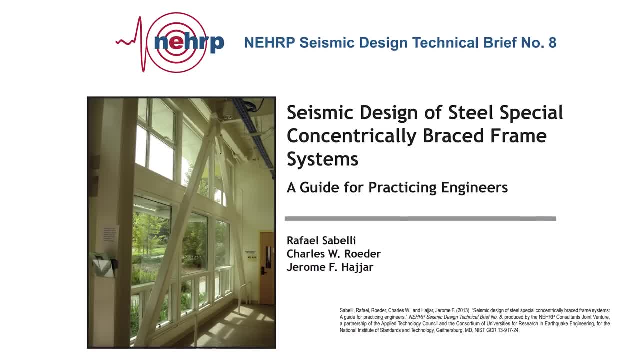 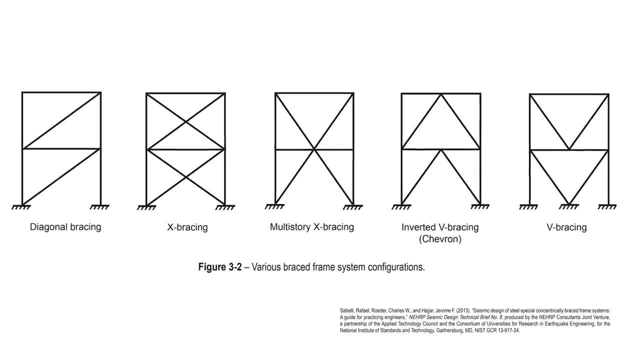 You can open up the floor plan a lot more with these. And number four are bracing systems. These are the bread and butter for steel buildings. Braces are stiff, strong and economical against resisting earthquakes, but they do get in the way of the architecture. Braces. 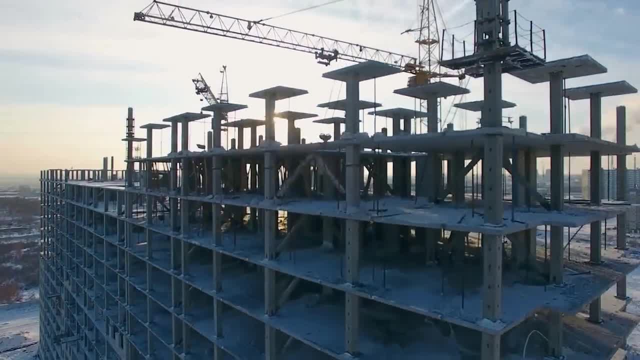 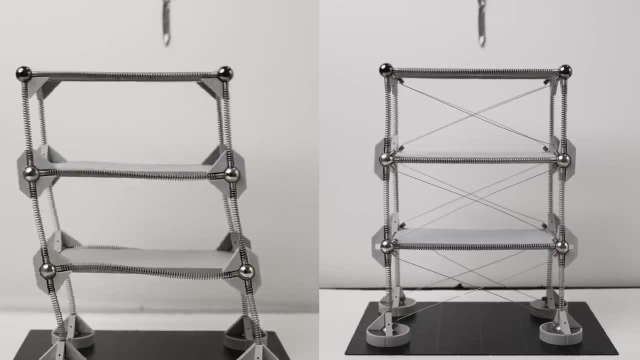 as the name suggests, brace the building during earthquakes and they are effective. If we install braces on the Mola model, you can see that during earthquakes they are stiffer and deformed less than the ones with the moment frame. And there is an engineering secret to using these braces. 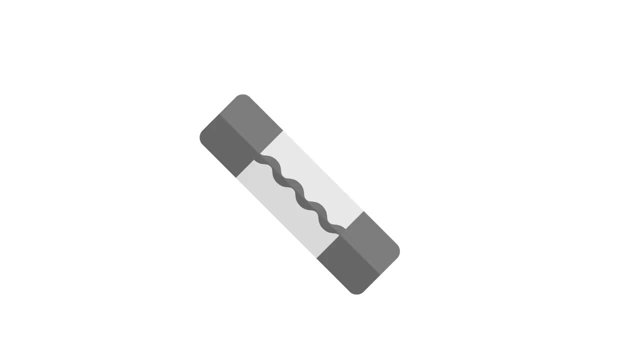 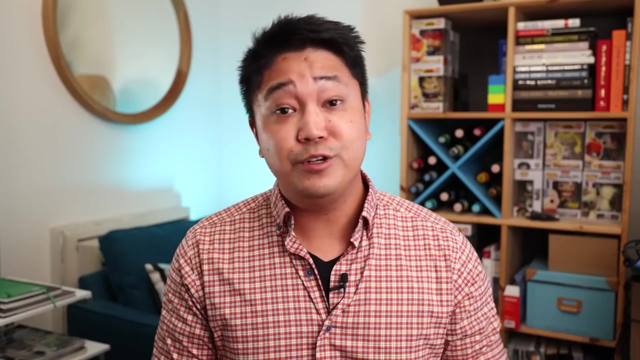 Structural engineers often design these braces as the fuse of the building during an earthquake event. Earthquake forces attack the weakest link in the building, and these braces are it. But don't worry, they're designed to take a beating. They're designed to be very ductile. 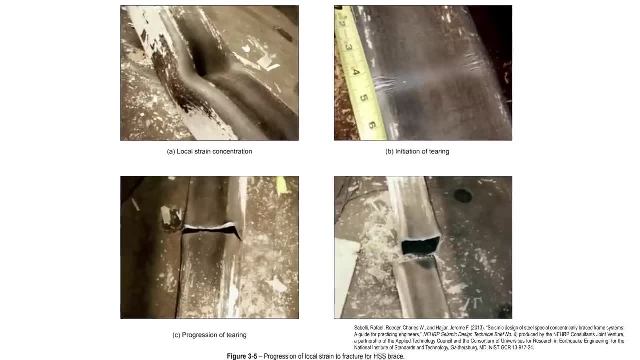 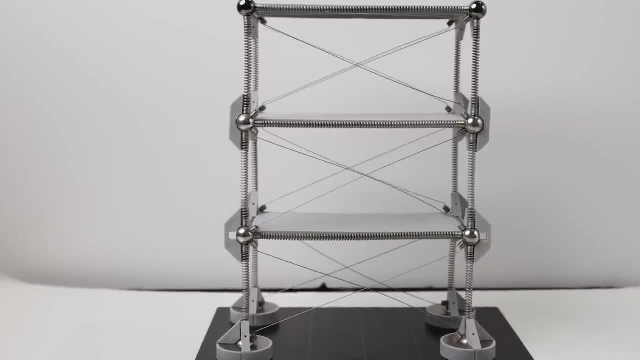 Basically, they can deform and get mangled without tearing apart, Similar to if you tried to mangle or split apart a paperclip. it's very hard to do. The earthquake forces focus all of their energy on the weakest link: the brace. 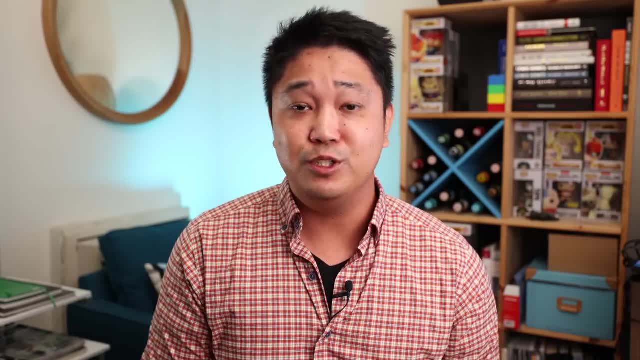 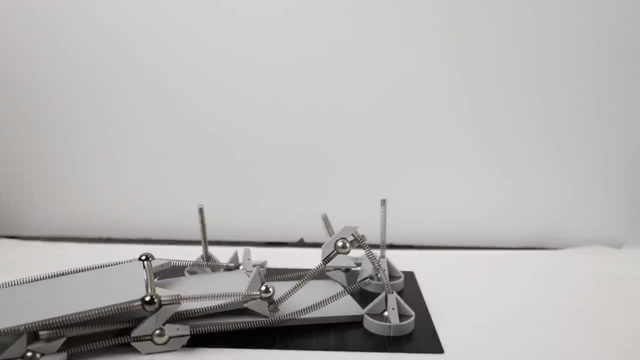 And that's good, because they ignore the most important parts of the structure, which are the beams, floor systems and columns. And trust me, you do not want the earthquakes attacking the columns. Number three are the shear wall systems. Structural engineers call them shear walls. 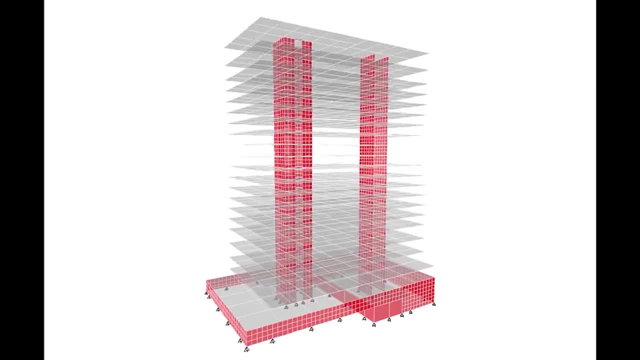 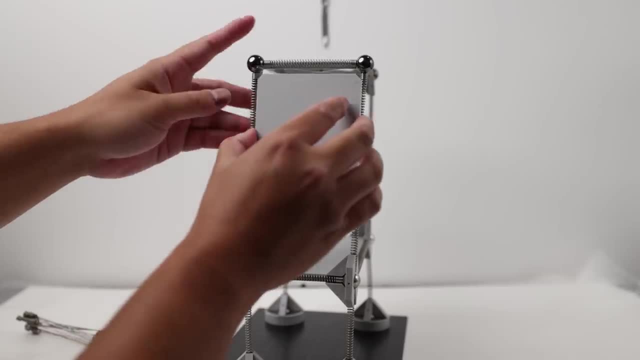 but they're basically walls that take the earthquake forces and they prevent the building from shearing off the foundation, And these are the bread and butter for concrete and wood buildings. When we install shear walls on the Mola model, you can see that these are basically the strongest and the stiffest of the 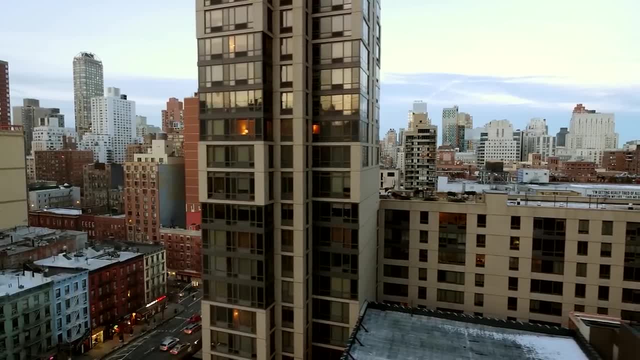 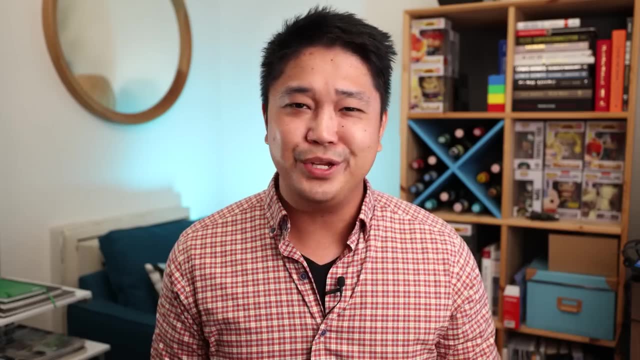 structural systems. So it's pretty common for you to see them use in mid rises and high rise projects. They're the most economical option to resist earthquake forces as well, but they're also the architect's worst nightmare, because it's a wall, I mean. 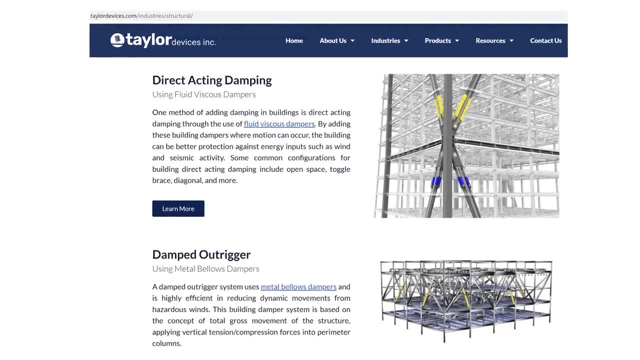 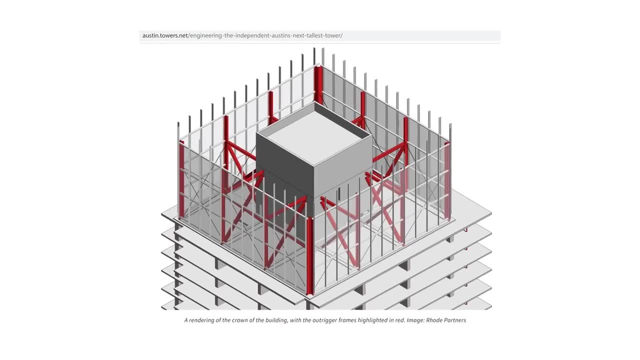 who wants to stare at a wall? Number two are dampers. Dampers reduce the earthquake vibration on the building or structure And there's various damper systems, such as liquid filled dampers, a mass tuned dampers or viscous dampers. 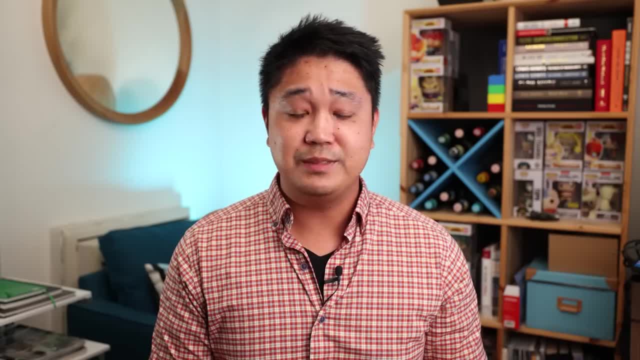 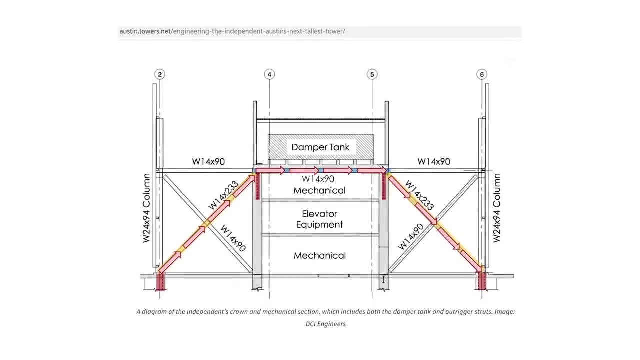 But for today let's focus on liquid filled dampers. Unlike the previous systems that we've been going over, this is not a brute force method system where bigger equals better. A real world application of this is a water tank filled damper placed on top of 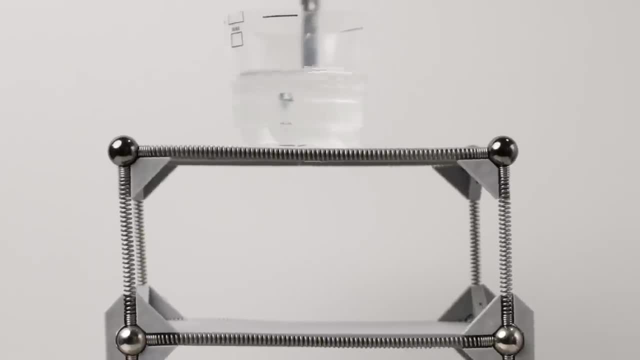 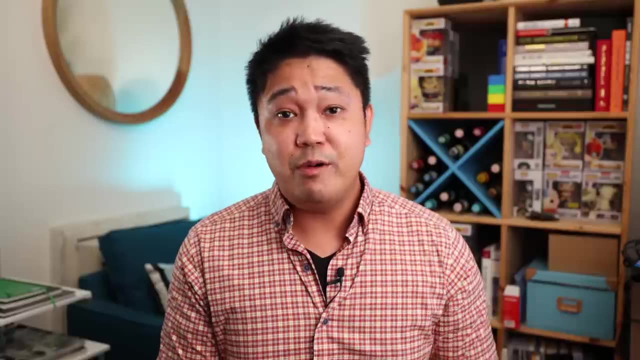 the building. The water sloshes around in the damper during an earthquake And this sloshing reduces the earthquake vibrations to the structure. Let's do this to our Mola model. First, let's see how it reacts to an earthquake without a liquid filled damper. 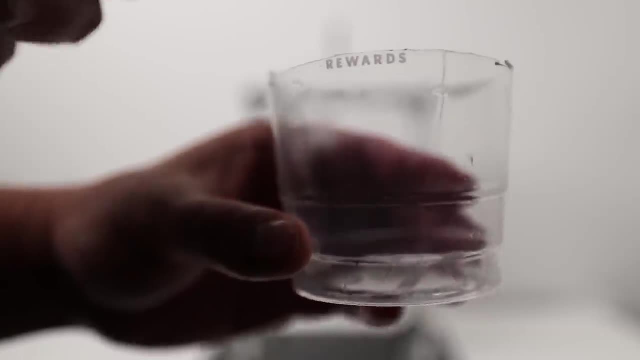 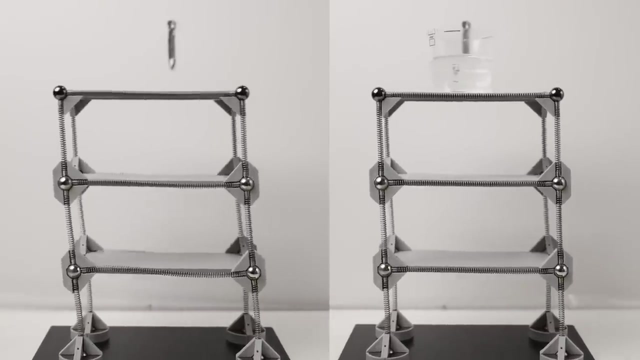 Now let's fill this damper up with water and put it on top of the structure, and let's put it through an earthquake. Comparing these two models, you can see that the water damper helps a lot with reducing earthquake vibrations, And number one is seismic base isolation. 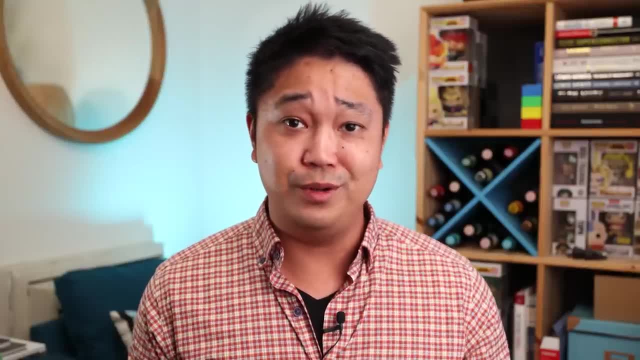 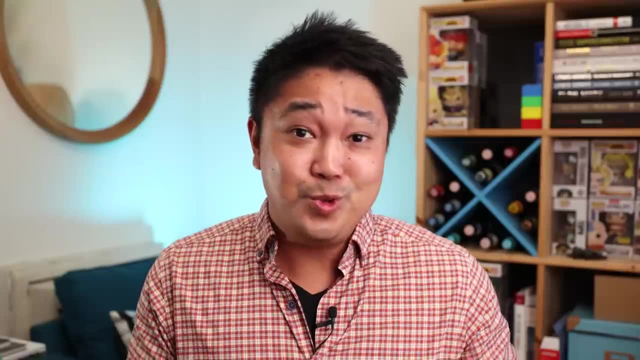 This method is probably the closest thing to earthquake proofing a building. This involves essentially putting roller skates under the building, So it's kind of floating above the ground. I mean, you can't get hit by an earthquake if you're not touching the earth. 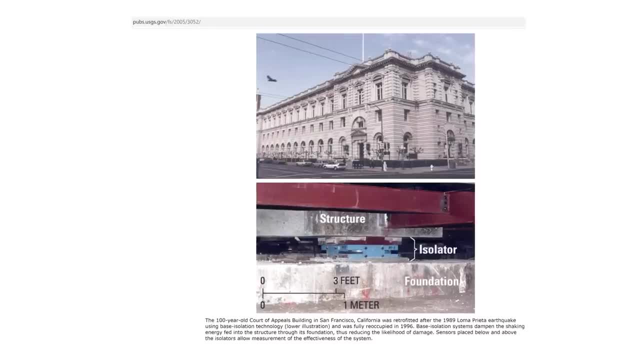 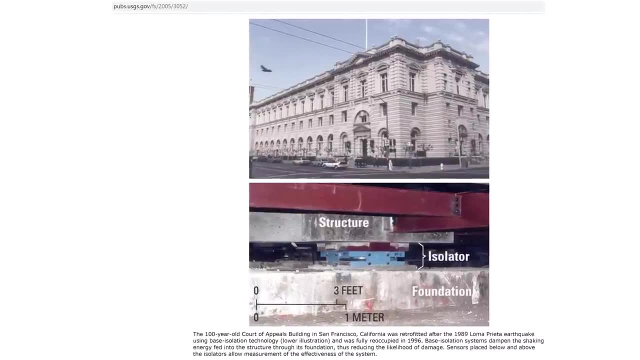 Huh, Real world applications of this involve putting these base isolators, which are usually in the form of a ball bearings, rubber bearings or friction bearings, underneath the structure. So let's see this in action with our Mola model. First, 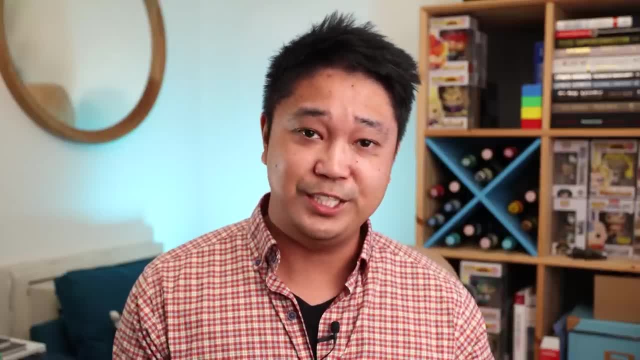 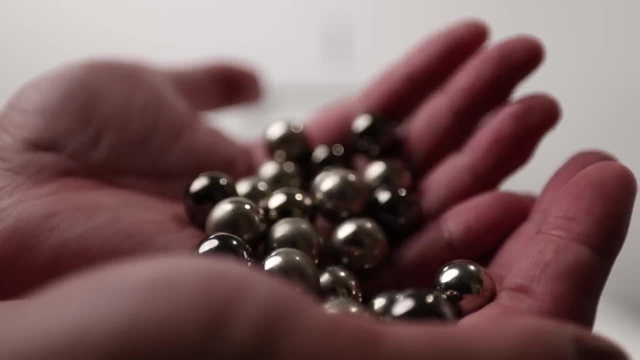 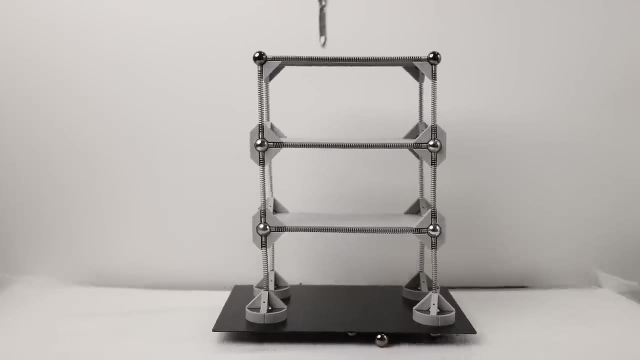 let's see how it reacts to an earthquake without base isolation. Now let's install the base isolation system. Here are some ball bearings. Let's put the building on top of those, So it's essentially floating and earthquakes. And here's the seismic base isolation system. 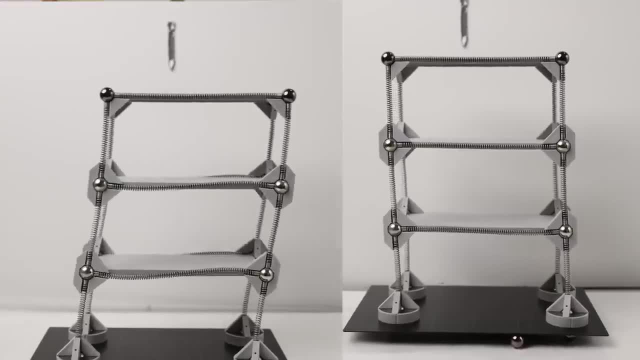 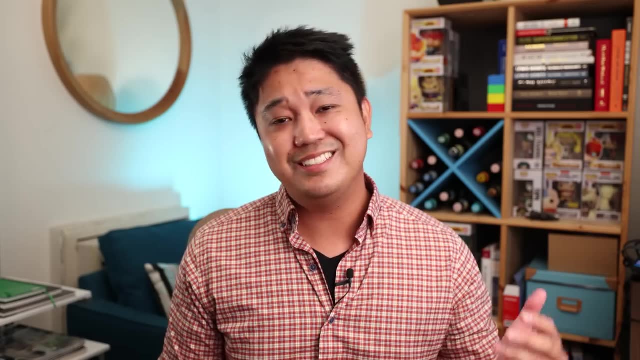 Comparing both of those, you can see how much base isolation helps- And I'm actually shaking the seismic base isolated structure a lot more than the un-isolated one. Unfortunately, this technology is still underused in most of the world, mostly reserved for high profile projects. 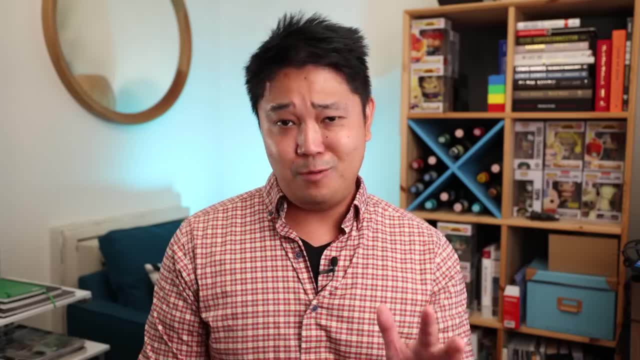 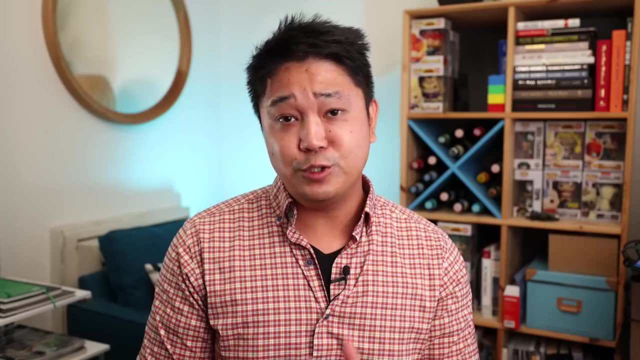 hospitals and historic retrofits. Now, if you want one of these Mola model kits, you can get 20% off any Mola product ordered at molamodelcom During the first week of this November by using my affiliate link in the description below. 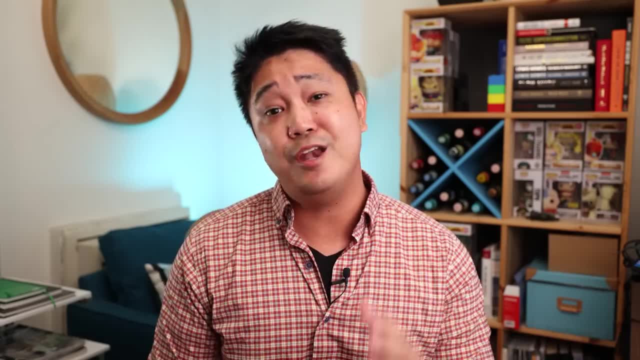 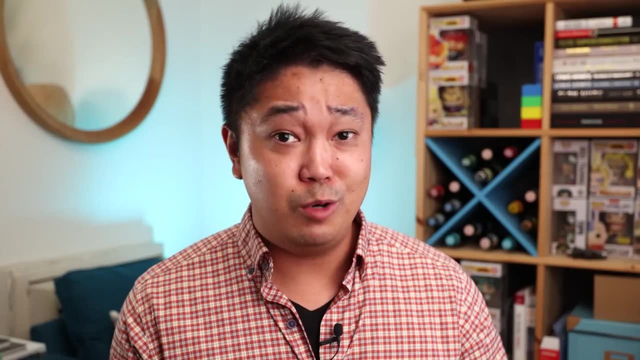 Note that this video isn't sponsored, but I do get a small commission at no cost to you. So if you want to help the channel, please consider using it, or don't just get it. They're really cool. I mean, check out my Mola model review video. 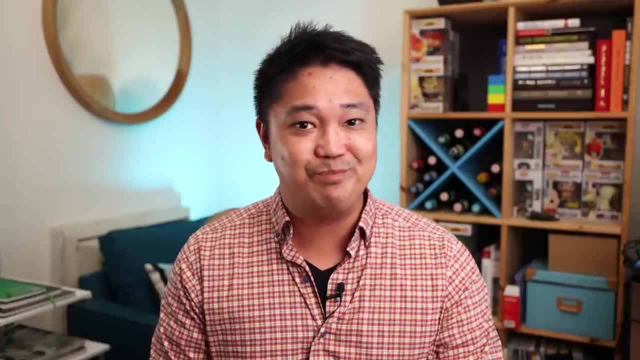 If you want to know more. thanks for watching and I'll see you next time. 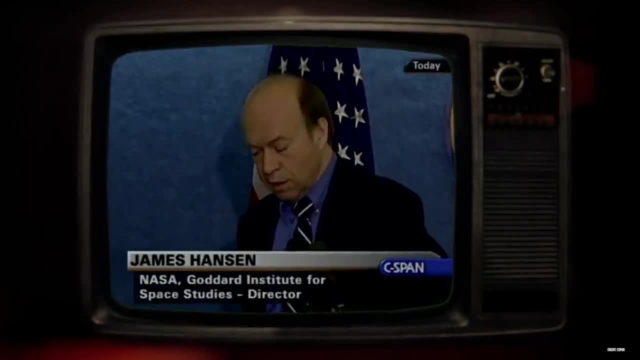 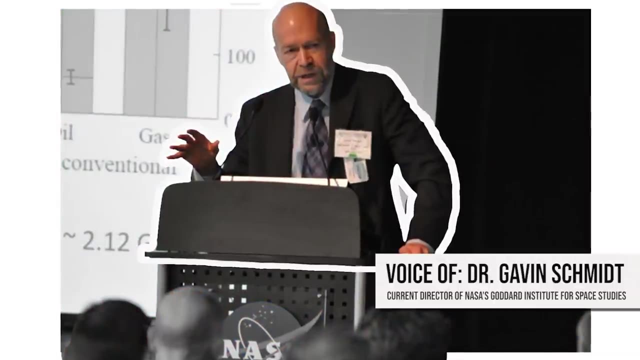 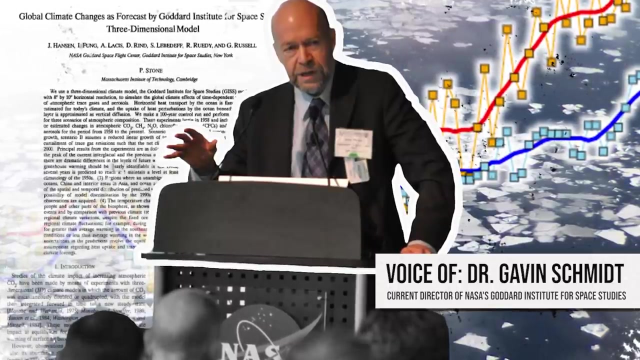 In 1988, Dr James Hansen, then director of NASA's Goddard Institute for Space Studies, stood before the US Senate and testified that Global warming has reached a level such that we can ascribe, with a high degree of confidence, a cause-and-effect relationship between the greenhouse effect and observed warming. 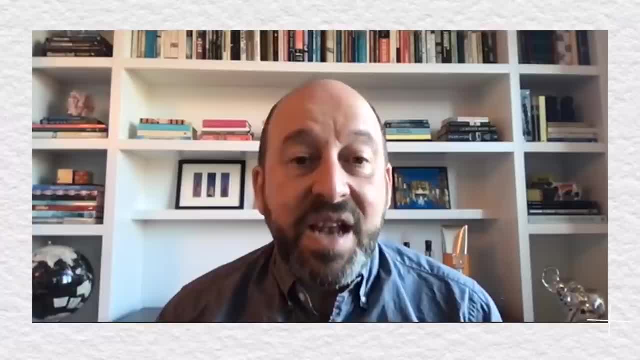 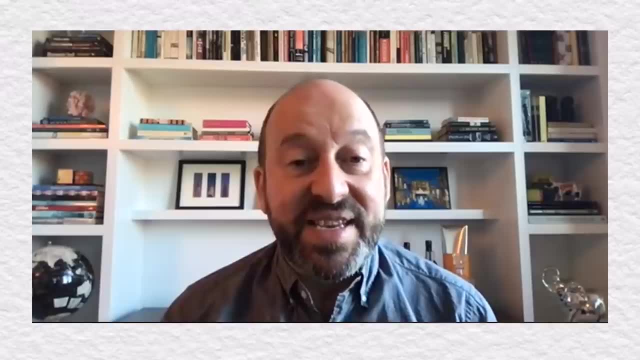 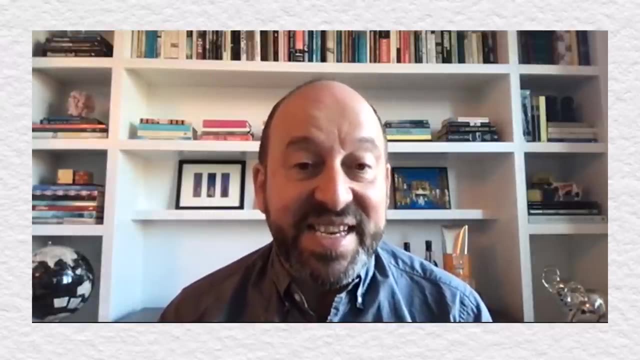 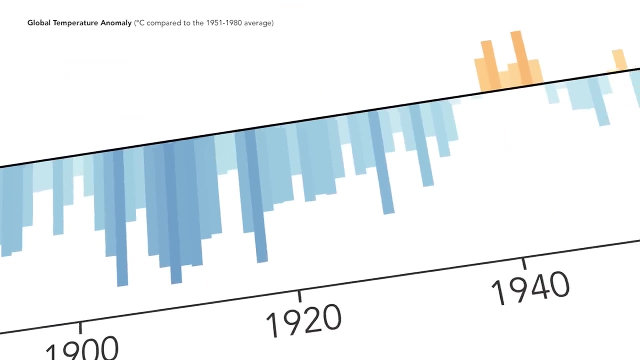 It is already happening now. This last year- 2021, comes in as the sixth warmest year on record, and it continues this large long-term warming that Jim Hansen was detecting even in 1988. And in 1988, that was also a globally warmest year, but now that ranks only 28th in the ranking. 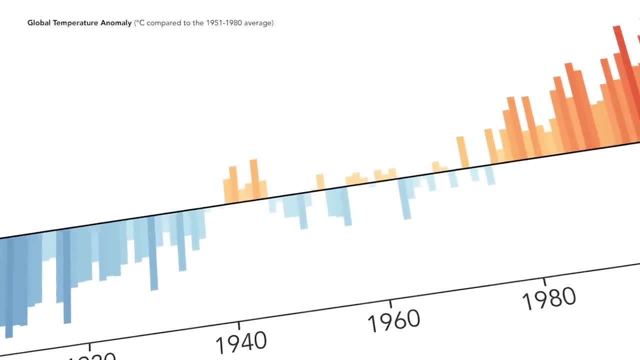 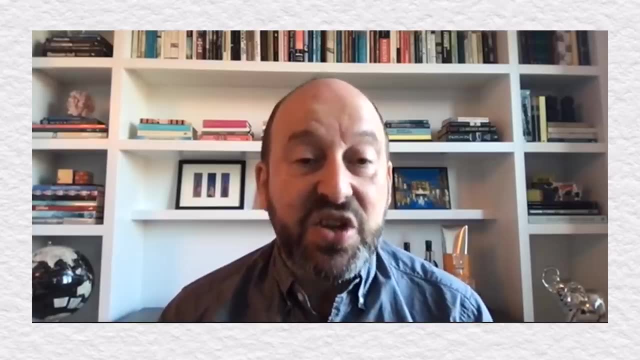 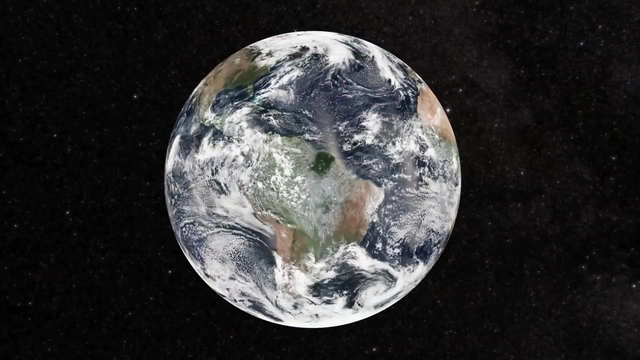 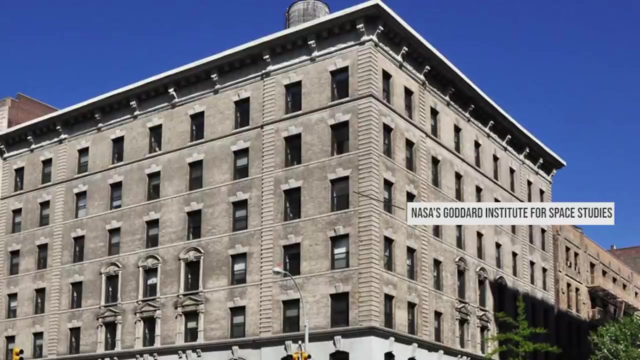 And so the warming that we've had since Jim Hansen's time in the US Senate- and observed warming- his testimony has been dramatic and totally vindicates the concern and the warnings that he put out at that time. The Goddard Institute for Space Studies, or GIS for short, maintains NASA's record of Earth's surface temperature called GISTEMP. 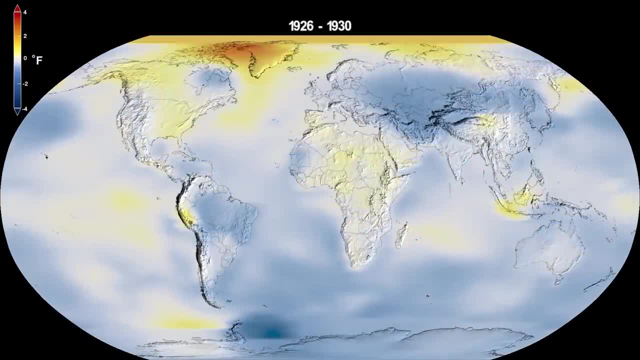 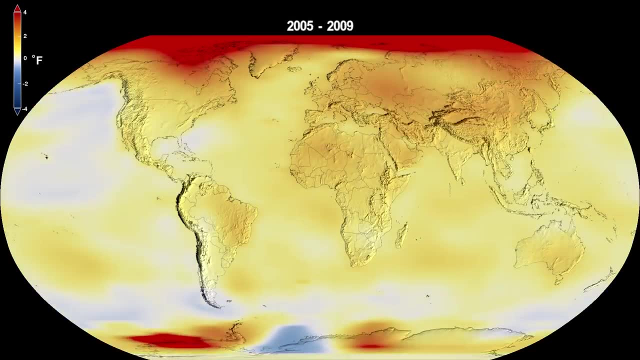 that shows a clear and unequivocal increase in our planet's temperature. GISTEMP stretches from 8.5 degrees Celsius to 8.5 degrees Celsius. This is 1880, long before NASA existed, until the present day. Now, when you think of NASA, you probably think of- well, space, right? 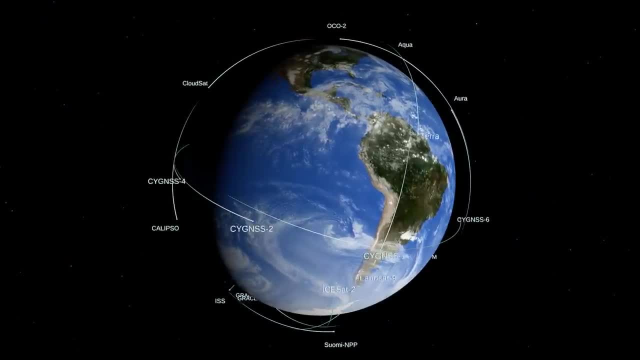 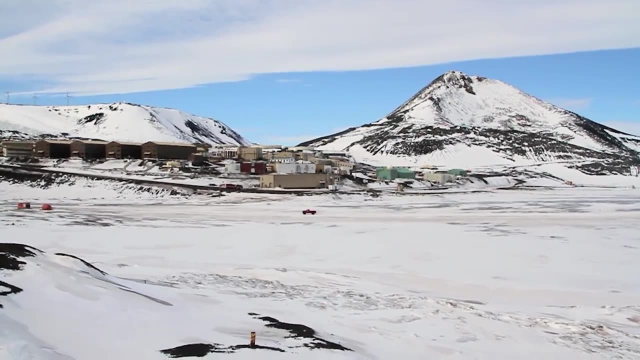 And we do lots of work studying Earth from above, But the GISTEMP record is actually built from the ground up. We collect measurements taken from weather stations, Antarctic research stations and ships and ocean buoys all around the planet to understand what temperature changes look like globally.